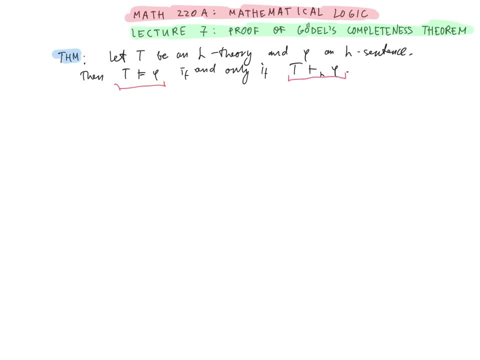 And on the right-hand side, we have a syntactic notion of existence of a formal proof, a syntactic object, a finite sequence of formulas which allows us to derive phi from T. Last time we have stated a reformulation of this theorem. 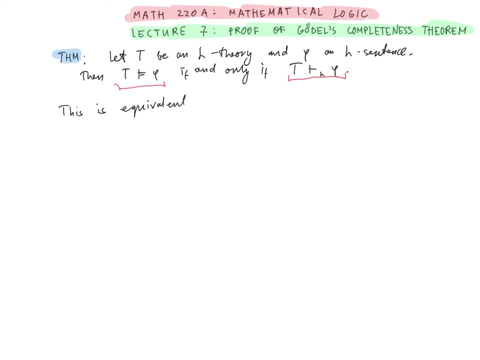 This is equivalent to the following statement: A theory T has a model of Godot's Completeness Theorem. It is consistent if and only if it is consistent. Last time we pointed out how to deduce the first result- Godot's Completeness Theorem- from this. 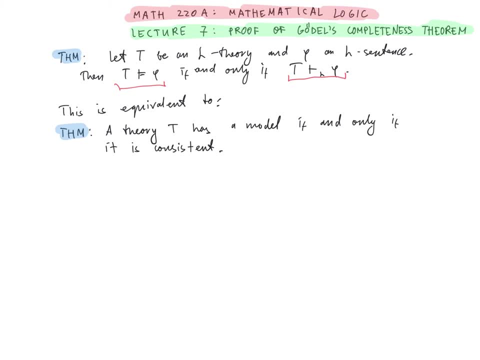 rephrased but equivalent variant, which again provides a connection between syntax and semantics. So existence of a model, a semantic notion, is equivalent to the syntactic notion of being consistent, that is, not being able to prove a sentence and its negation simultaneously. 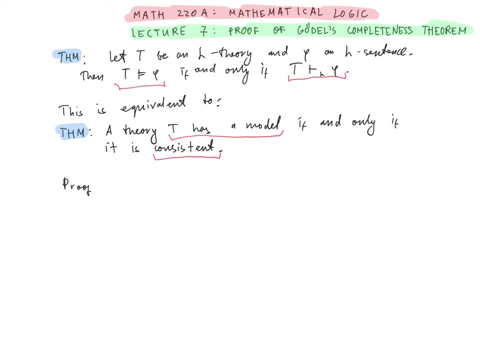 Let's begin working towards the proof of this theorem. The easy direction- If T has a model, then it is consistent- is already proved, Indeed by the soundness of our formal proof system. we know that if T proves phi, then also phi is a logical consequence of T. 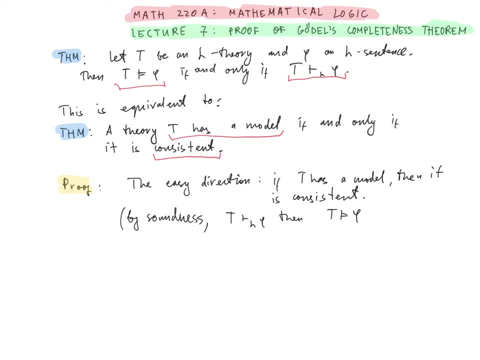 Now, if T was inconsistent, we would also have some sentence so that its negation is provable as well, in which case we would have that T has the negation of phi as a logical consequence as well, but by assumption T has a model. so if A is a model of T and both phi and not phi are the logical consequences of T, 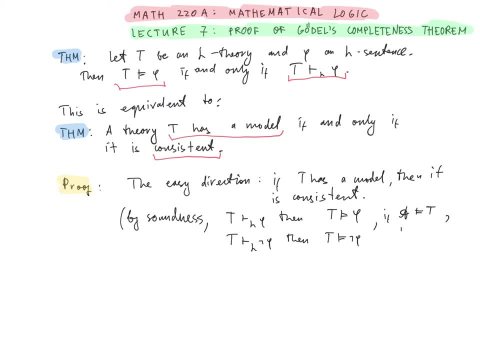 we must have that A satisfies phi, but also that A satisfies the negation of phi, and this is of course impossible by the definition of satisfaction of formulas. So this gives us the easy direction. Hence our task is to show the opposite direction. so we need to show that any consistent theory T has a model. 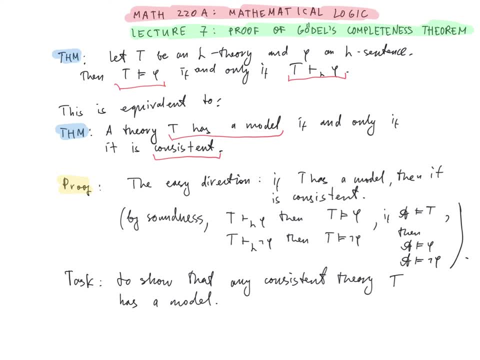 The theory of T has a model. In order to prove this direction, The theory of T has a model, so we need to show that the theory of T has a model, prove this direction. we will use the so-called hankins method of building. 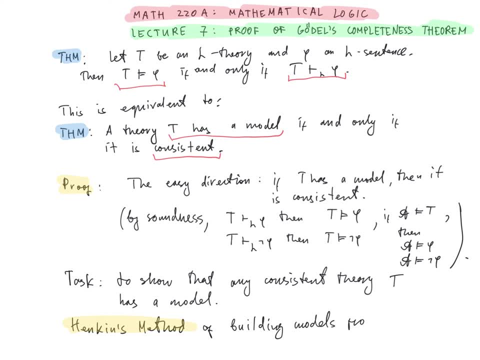 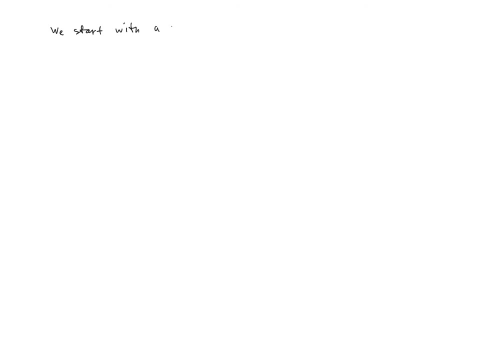 models from constants. we start with the consistent theory t in a language l, in order to build a model for it. we will define a certain expansion, t plus- of t in some language, l plus extending the language l with better properties towards this. let us start with the definition of what better properties we are talking about. 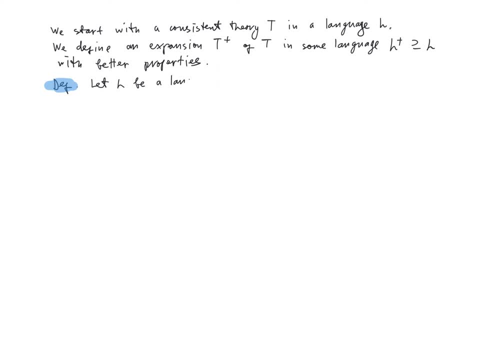 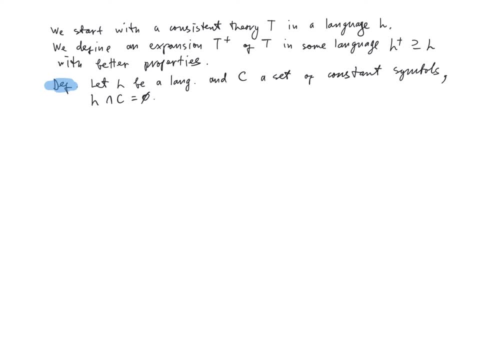 and not contained already in the language L, Then we will say that an L union C theory T plus admits Henkin witnesses in C. if for any L union C formula phi of C of X with a single free variable X there exists a constant symbol, little c. 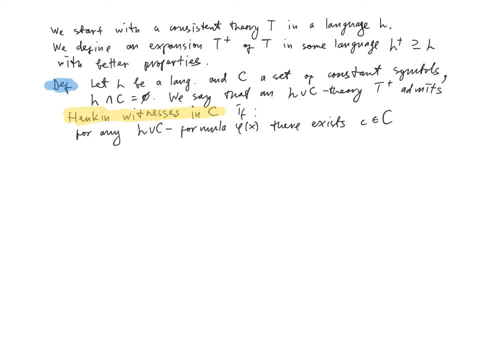 in our set of constant symbols, capital C, such that the sentence exists X, phi implies phi, with C substituting X belongs to the theory T plus The idea of this definition as to ensure that every time we have some existential formula, the formula exists X, phi, then. 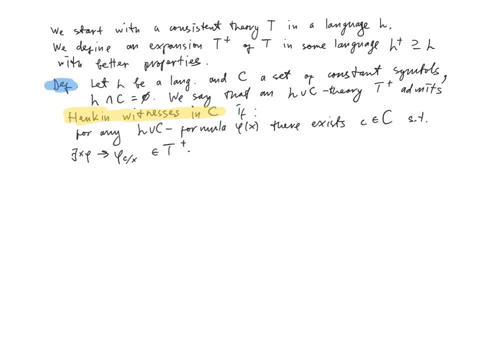 it is always possible to find a witness for it, so namely an element such as phi, which is given by the interpretation of some constant symbol. So that's the intuition behind it. Now, if A is an L structure and the set A the base set of the structure, 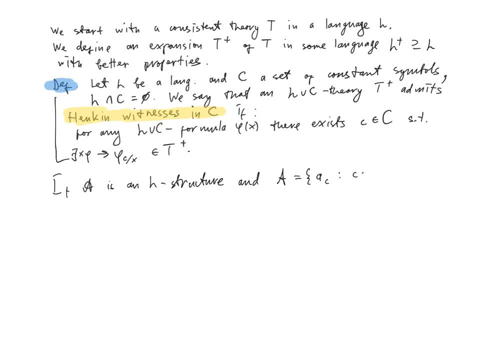 is given by A, C with C, a constant symbol from the set capital C. So if this is an enumeration, possibly we can write it in the set C as an enumeration, We can write it in the set C. So if this is an enumeration. 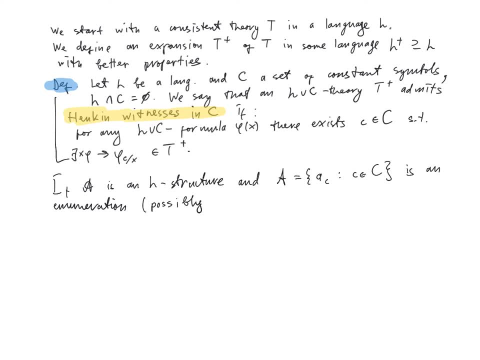 So if this is an enumeration, We can write it in the set C as well, possibly with repetitions, so possibly not injective of its base set by C. So what we mean by this is that it's possible that the same element of the base set 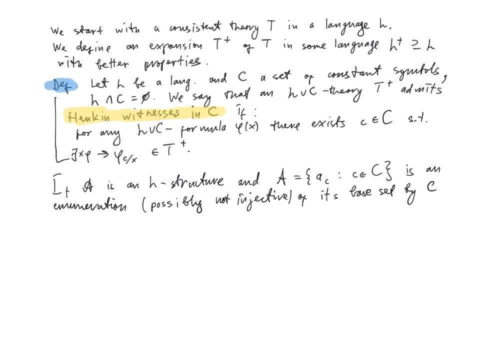 is of the form AC for multiple constant symbols, Then we denote by A+ the structure in the language L, union C obtained from A by interpreting the constant symbol C by the element AC. Then we can consider the theory of the structure A+, which we already know is a complete theory. 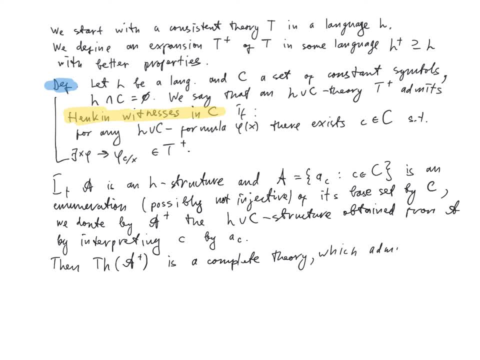 which, moreover, admits Hankeen witnesses in C. So this tells us that, given any structure and a bunch of constants naming the elements of the base set of this structure, if we add all of these constants to the language and consider the complete theory of this expansion A+. 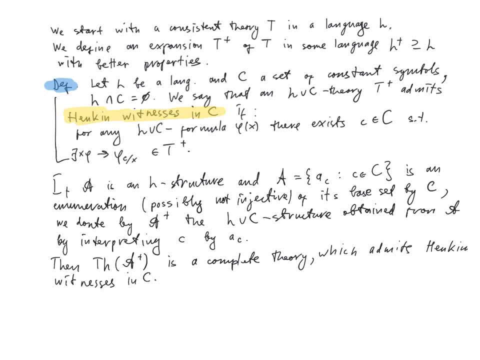 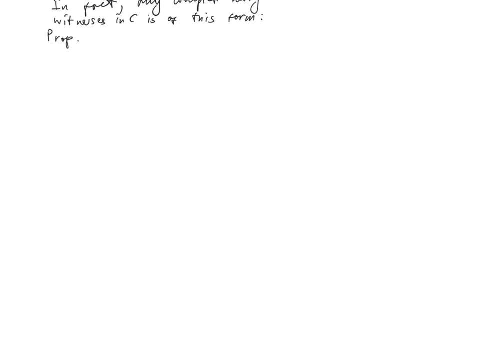 which of course is complete, it is automatically going to admit Hankeen witnesses in C. Turns out that any complete theory which admits Hankeen witnesses in C in C is already of this form as well, namely proposition: any complete L union C theory T+ which admits Hankeen witnesses. 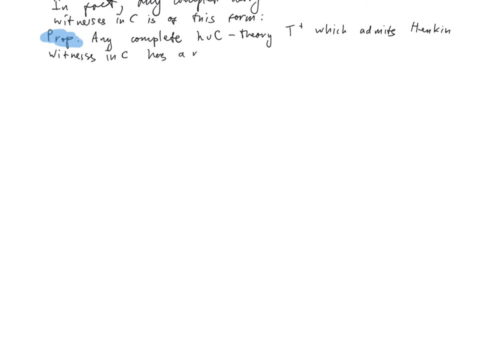 in C has a model A+ consisting of L union C theory T+, which admits Hankeen witnesses in C has a model A+ consisting of of constants of C, That is, with base set A plus given by the interpretations of the. 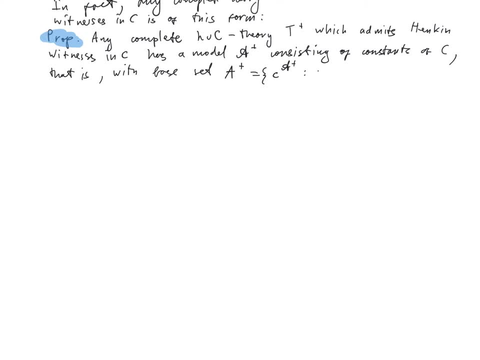 constant symbols C in A, plus for all the constant symbols C in the set capital C. Let's call this proposition 1, so proof of proposition 1.. First note that replacing the theory T plus by the set of L union C sentences phi, such that T plus proves phi. 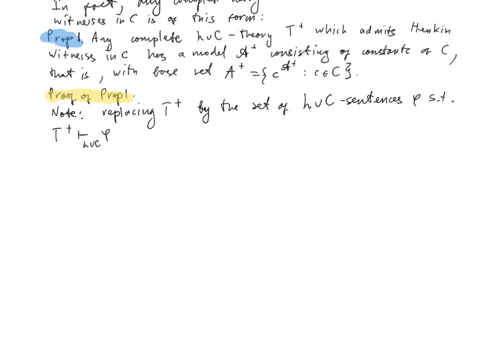 in the sense of the language. L union C does not change the assumptions. Indeed, all of the sentences required by the definition of admitting Henkin witnesses are already in T plus and we are only adding more sentences, and also the same, for completeness. 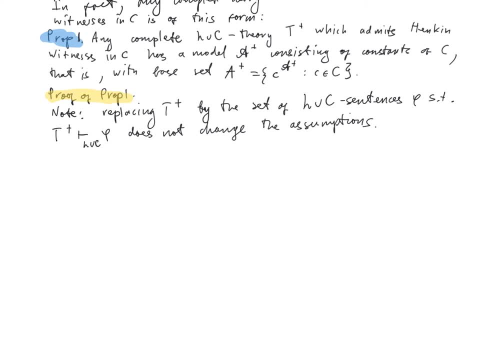 So T plus is already complete, so it already proves either phi or the negation of phi for every L union C sentence, T sentence phi, And so the same is going to hold for any larger collection of sentences than T plus, And so we may assume that T plus is what is called deductively closed. 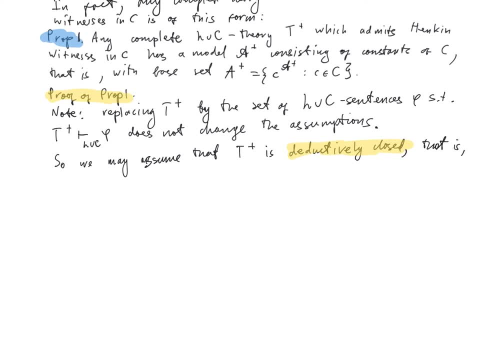 That is, we have that T plus proves phi in the sense of the language L union, C if, and only if, phi belongs to T plus. Given a pair of elements- C and D- from the set of constant symbols C, we will write: C is equivalent to D. 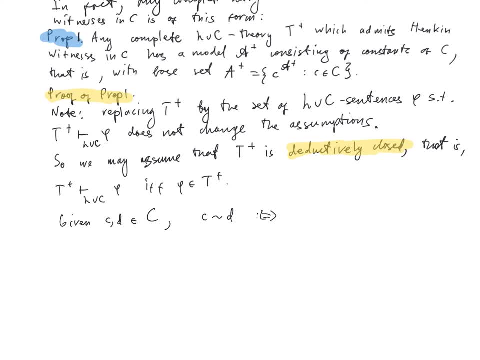 When C equals D is a sentence belonging to T plus. So note, this is a well-formed sentence in the language L, union C. then it follows from the equality axioms That this defines an equivalence relation on the set of constant symbols, C Namely. the equality axioms express that the equality 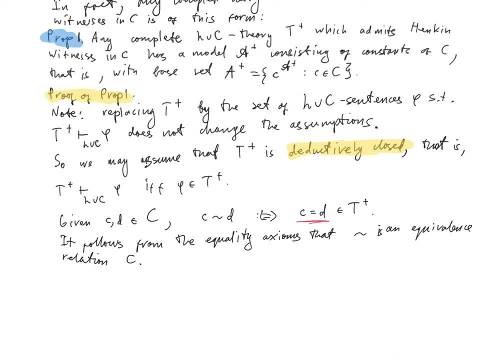 axiom L is transitive and symmetric and reflexive, and hence each of these properties is provable from T plus, and so, by our assumption of deductive closeness, it belongs to T plus as well. So we get that this is an equivalence relation. 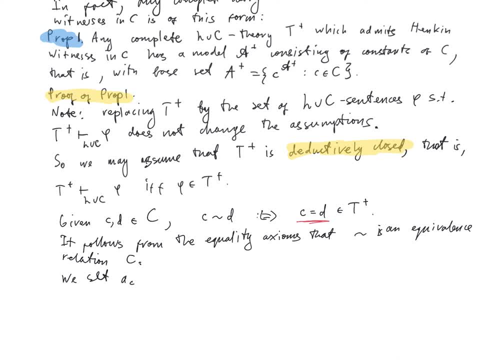 We set AC equal to T plus, So we get that this is an equivalence relation. We set AC equal to T plus, So we get that this is an equivalence relation. We set AC equal to T plus. Lay out these values of this set to be the equivalence class of the constant symbol C. 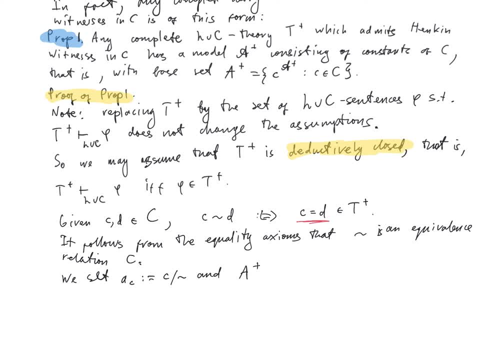 And we define the set A plus to be the collection of all of these equivalence classes, AC. So we choose a value of guaranteed scholars, AC, and we take the constant symbol from the set C. Then we have that the set A plus is non empty. The set is großen. So now the relation with A plus C is non empty. Now that studying this will likely answer one more question: And what should we do if we were changing to different classes? We should try to have more semblance, pequeness to it. 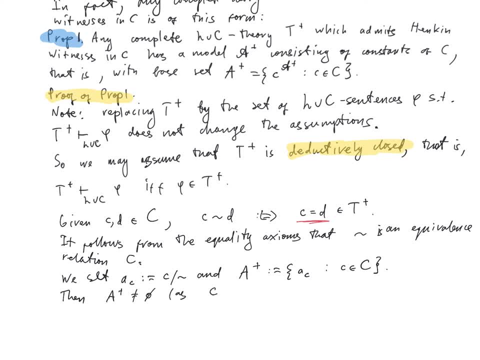 So let's see what we can do. accordingly. I'd like to understand the equation that Joe Andasu said in the first part, as clearly the set of constant symbols C is non-empty by the assumption of admitting hanking witnesses in it. then we define an L union C structure A plus. 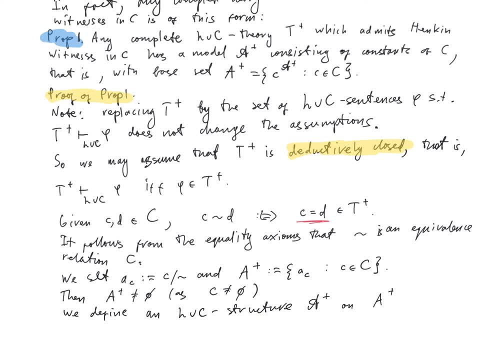 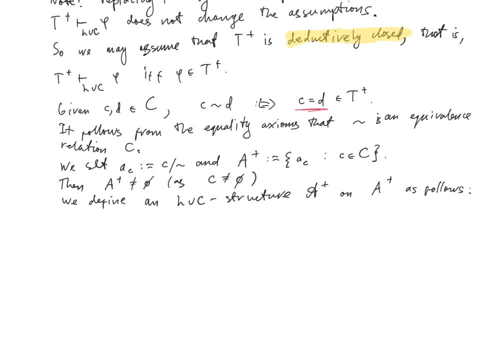 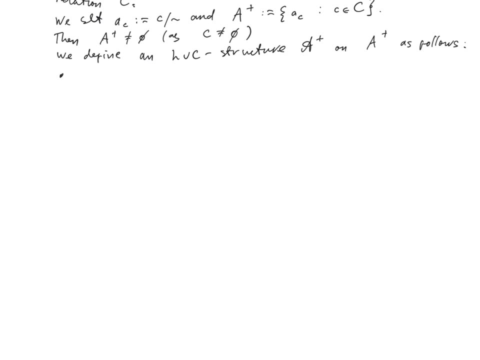 on this underlying base set A plus as follows: First for D, a constant symbol, we set the interpretation of this constant symbol in A plus to be the element AC. if C equals D is a sentence in T plus where C is some element of the set of constant symbols. S Note that such a 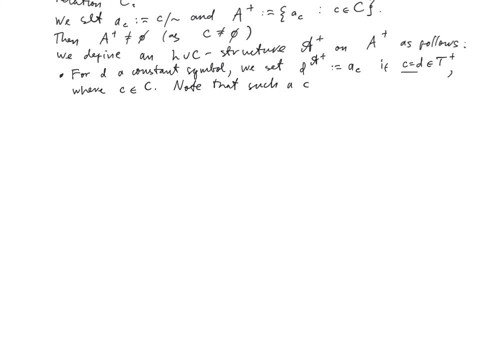 constant symbol in C in satisfying this sentence always exists by assumption of admitting hanking witnesses in the set capital C. Indeed, we have that D equals D implies exists. x. x equals d is a sentence in t plus by the second quantifier axiom. 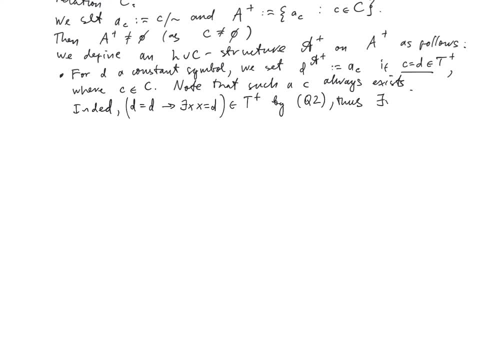 and thus we also have that exists x, x equals d is a sentence in t plus. by the modus ponens rule and the assumption that t plus is closed, under deduction, And since t plus admits Henkin-Witnesses and C, there exists some constant symbol C in the set capital C, such that exists x, x equals d. 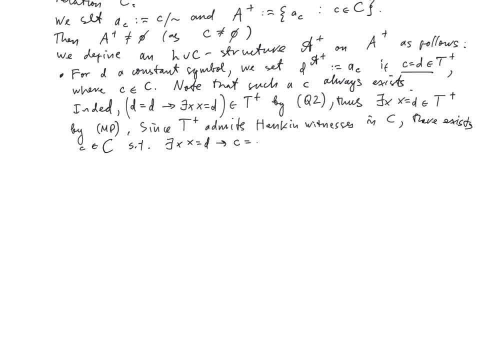 implies C equals d. this whole formula is in the theory t plus. so by modus ponens again we have that C equals d is a sentence in t plus, as wanted. Note also that axioms, the element which we defined to be the interpretation of D, does not. 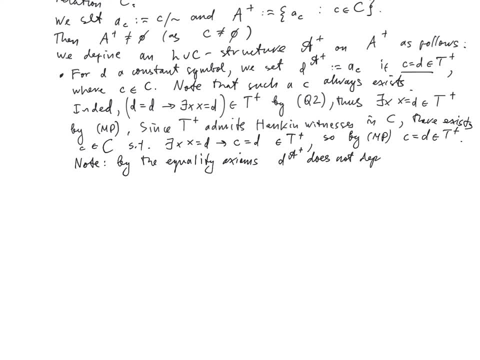 depend on the choice of C, since this interpretation is well defined. Next, we define the interpretations of the relation symbols. So, given R is a relation symbol of RAT n from the language L, So we define the relation symbols of RAT n from the language L. 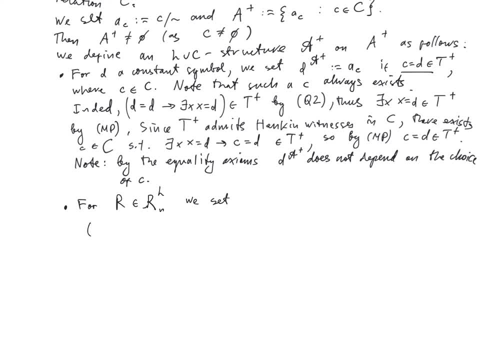 So we define the relation symbols of RAT n from the language L, We will set the interpretation as follows: So we will say that a tuple AC1, ACn from the base set A+ belongs to the interpretation of this symbol in the structure. 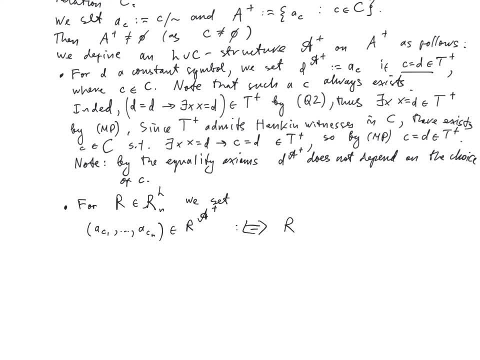 So we define it to happen if, and only if, the sentence R, C1 through Cn belongs to the theory T+. This relation is well defined by the equality axioms, namely E5, which contains axioms expressing that the equality symbol is always interpreted as a congruence. 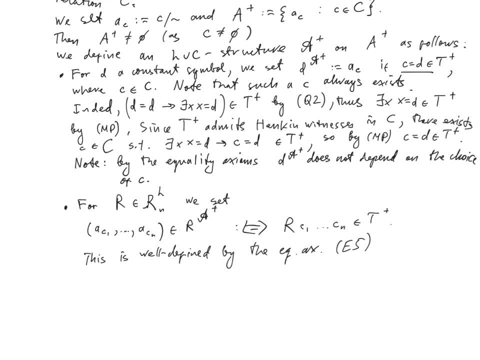 for the expression T+ For any relation symbol, And so, by deductive closure, this is again in T+ and guarantees that this is well defined on the classes, even though we are talking about representatives of the classes here. Now for function symbols. 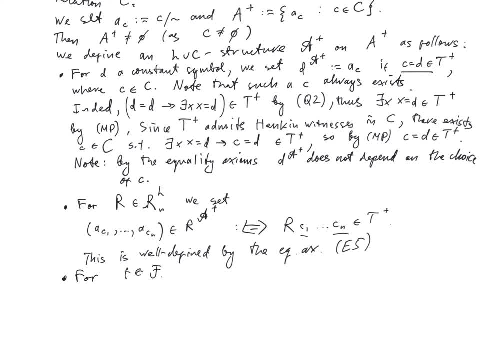 we have that given F a function symbol of R T, N in the language L, we set the interpretation of F in the structure A+ on a tuple, AC1 through ACn, to be equal to AC0, if, and only if, we have that the sentence F, C1 through Cn. 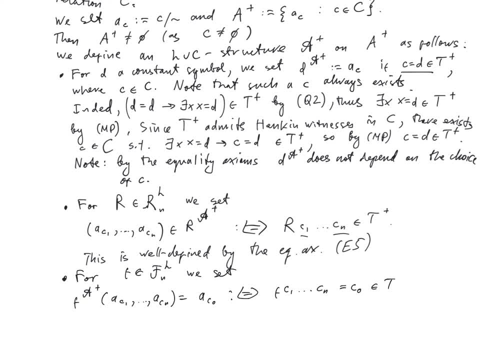 equals C0, is, in the theory, T+. Now, this is well defined by the equality axiom E4, which expresses that the equality relation is a congruence with respect to any function symbols and also, as in the case of constant symbols. 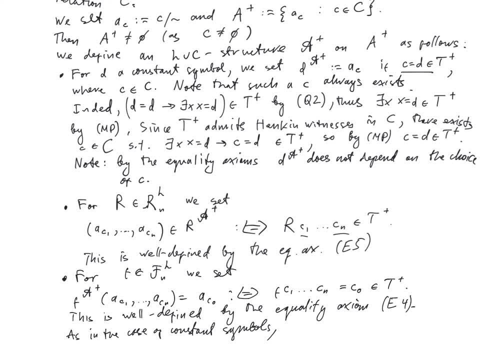 using the fact that T plus admits hand, can witnesses and is deductively closed, we can show that the function F A plus is everywhere defined and is indeed a function. This way we have defined all of the non-logical symbols on the underlying base set A plus. 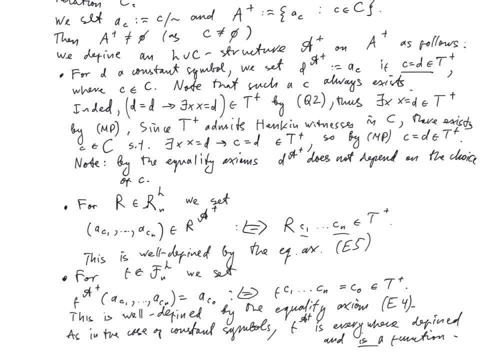 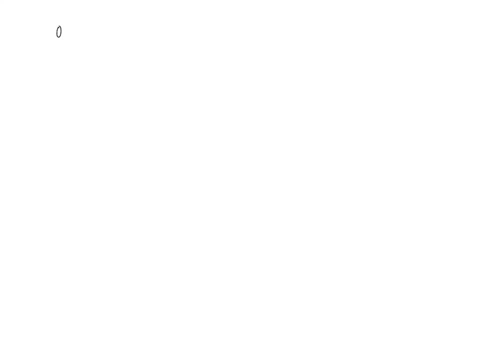 consisting of the equivalence classes of the constants and have demonstrated that, indeed, curly A plus is an LC structure which is well defined. Then we have the following observations: One, if T is an L union C term without variables and little c, 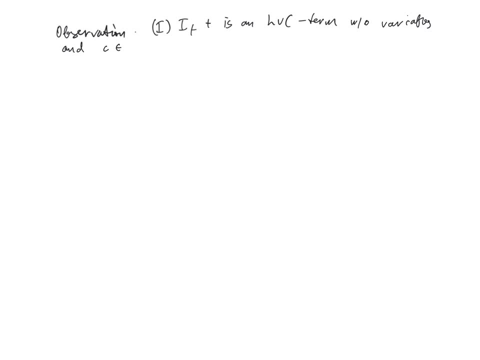 we have the following observations. One: if T is an L union C term without variables and little c as a constant symbol includes set C, then we have that the interpretation of this term in A plus is equal to AC, if, and only if, the sentence: 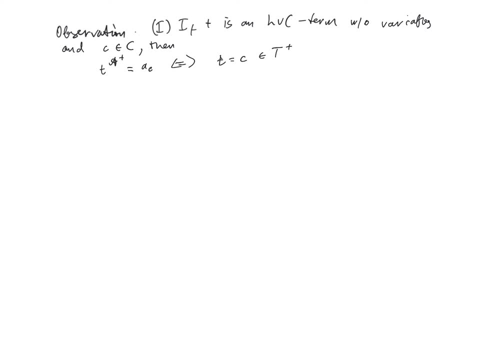 T was equal to C is in T plus, and the second claim lets E, b and L, c be to T union C sentence. then we have that A plus satisfies Psi if, and only if, Psi belongs to T plus. So these two observations tell us that the 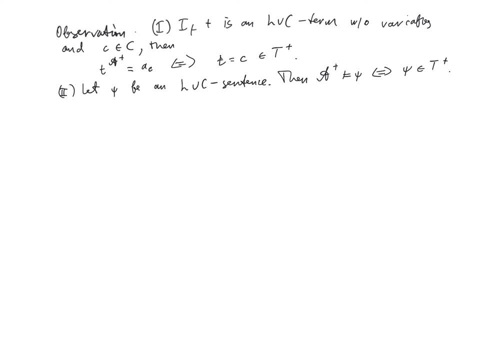 satisfaction in the structure A plus is completely controlled by which sentences are in T plus In particular. this second observation is going to be sufficient to conclude the proof of the proposition, because every sentence Psi in T plus is going to be realized in the structure A plus, and so, in particular, we have that A. 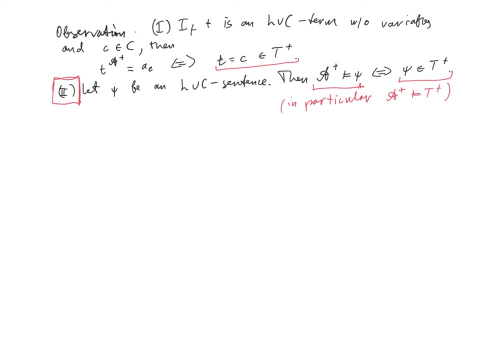 plus is a model of T plus, which is the desired conclusion of the proposition. So let's prove these observations. Item 1 follows by induction on the height of the term T. The case of height 1 is given from the definition of A plus. so the interpretation. 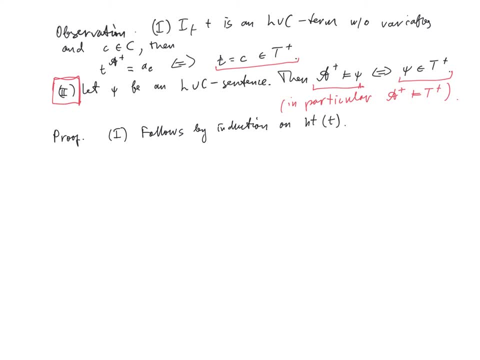 in the case that is a term or a constant. the definitions of the interpretations in A plus guarantee that this holds. this equivalence holds because that's how they were defined on the left hand side, using the condition on the right hand side and the inductive step. 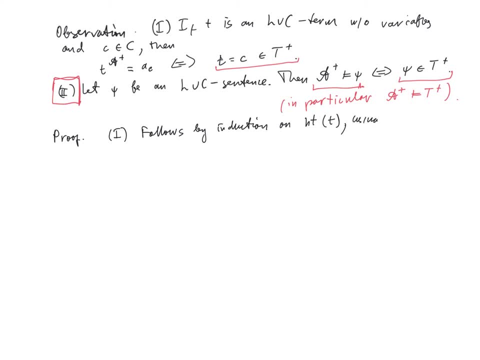 one uses the equality axioms for composing several terms with each other. so this is part one, and for part two we again argue by induction on the height of the terms of the formula psi. also recall from our early discussion of simultaneous substitution in the previous lectures that the height of any sentence psi. 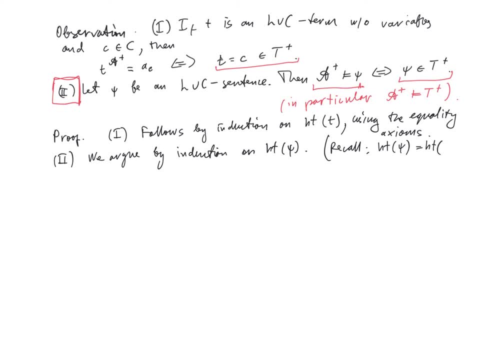 is equal, or a formula psi is equal to the height of the formula psi, with the tuple of terms as bar substituting the tuple of the variables x, bar. so now we begin with the base case. if psi is of the form, t1 is equal to t2. 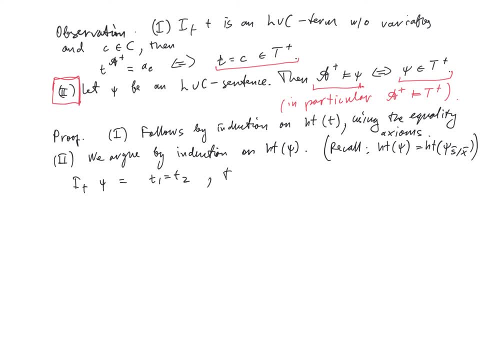 for some terms t1 and t2, then 2 follows directly from 1. so this is the base case. next, if psi is of the form rt1 through tn- for some terms t1 through tn- and the relational symbol r, we choose some constant symbol ci. 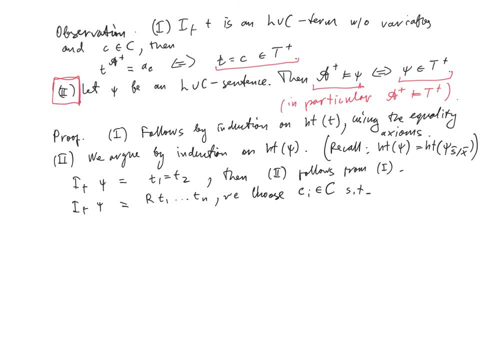 in the set capital C, such that the interpretation of the term ti is equal to aci and the interpretation of the term ti is equal to aci. of course, since psi is a sentence, there are no variables involved in any of the terms, so this interpretation just gives us an element of the base set. 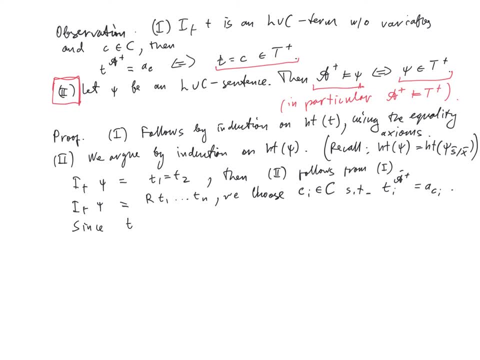 now, since we have ti equals, ci is a sentence in t plus. we also have that a plus satisfies psi if, and only if if, r c1 through cn is a sentence in t plus. if, and only if, psi is a sentence of t plus. here the first equivalence. 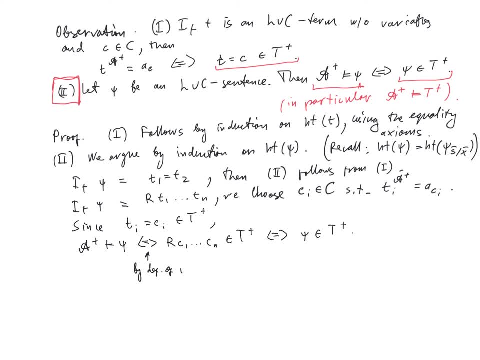 follows from the definition of the structure a plus, and the second sentence follows from the equality axiom if, and only if, E5.. Next case is: if Psi is equal to the conjunction of Phi1 and Phi2 for some formulas of Phi1 and Phi2 of smaller height, then clearly 2 for Psi follows. 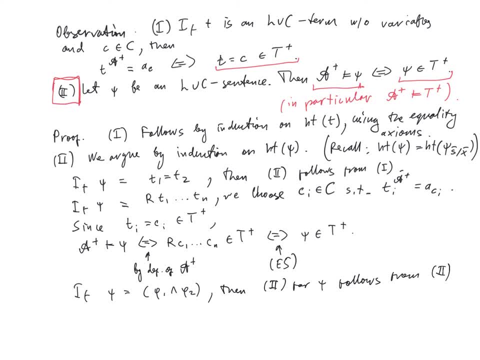 from 2 being satisfied for both Phi1 and Phi2.. Next case: if Psi is equal to the negation of Phi, then we have A plus. satisfies Psi if, and only if, A plus does not suffice. satisfy phi just by the definition of satisfaction in a structure, if, and only if, phi is not. 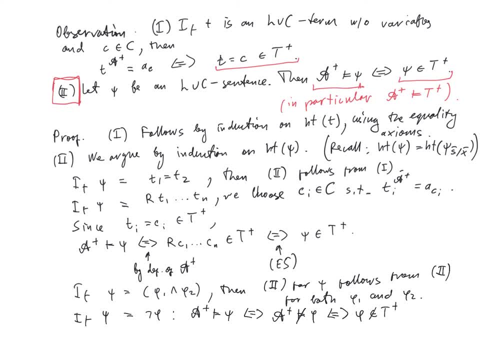 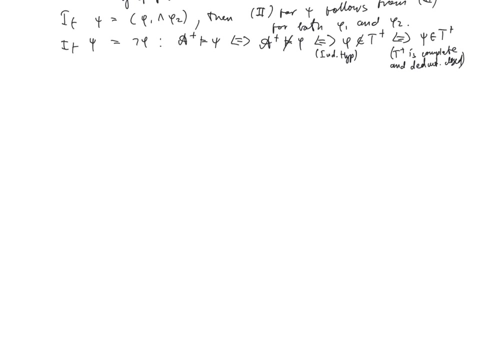 in T plus by the induction hypothesis, since phi is a formula of smaller height, and this holds if and only if, phi belongs to T plus, since T plus is complete and deductively closed. Finally, we have to treat the case when the formula 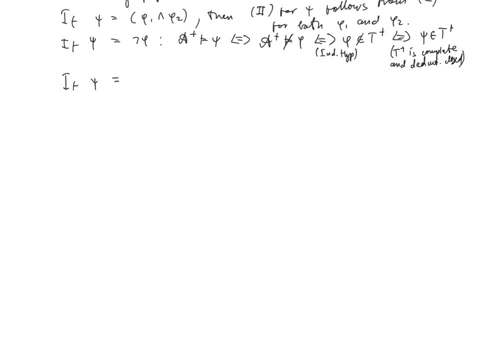 Psi is of the form exists for some formula, phi of smaller height- In this case note that Psi belongs to T plus if, and only if, there exists a constant symbol C in the set of constants, capital C, such that the formula, The kernel for a re- quote, Freeze where the function is. 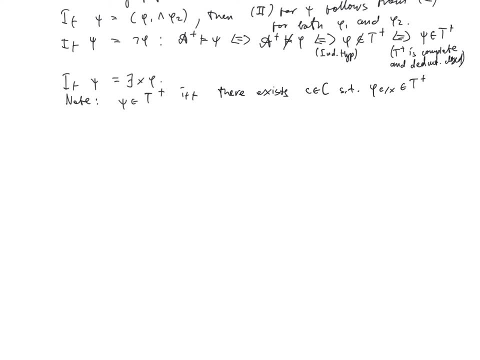 C substituting x is in T plus. Indeed we, assuming that T plus admits bra kannke and witnessers in C. Hence the only if proof of non-B. First G equipment in the set of constants. In this case, here a max if, and only if, cell of labor is in result c, then the maximum value. of C have an index in result can be reduced as x. Variety of statements in this class. darlingiels. He wrote about condition Europata isenneus. This, what rubric. which participants would any Cake? this read also: in C data are organized for飛duck took us into the prism in which there's limits. 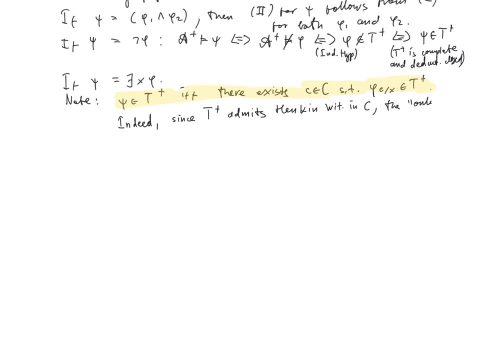 At least the norm: 요робик максимal y ussuر на. е versuchen иír в пр términе. if part follows, and for the if part we can use the quantifier axiom q2, which tells us that phi with c substituting x implies exists x. phi is a universally valid formula. 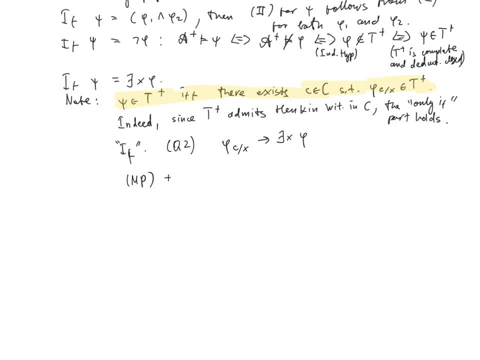 So by modus ponens and deductive closure of t plus, we conclude that the formula exists: x phi belongs to t plus, which is the desired conclusion. Using this we have: A plus satisfies psi, if, and only if, A plus satisfies psi, If A plus satisfies phi of AC for some constant symbol c in C by the definition of satisfaction. 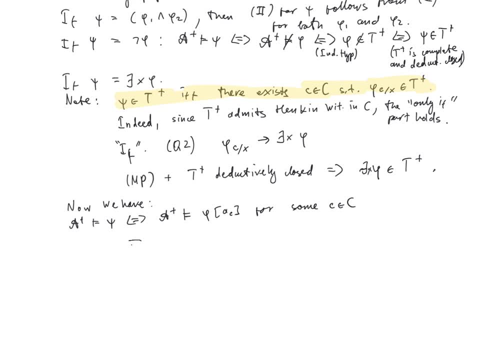 for an existential formula in a structure. now we have that this holds if, and only if, A plus satisfies phi with c substituting x for some constant c in C. So this holds by the substitution lemma. Now this is equivalent to the condition that phi with c substituting x belongs to t plus. 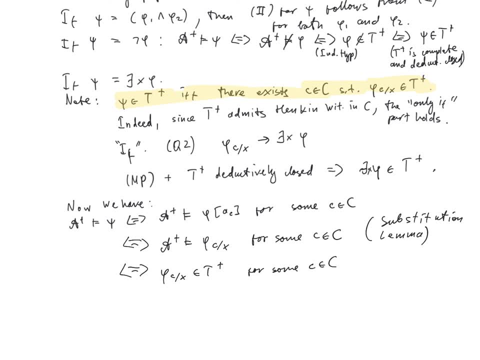 for some constant symbol c in the set capital C. So this is part of the induction hypothesis. since the height of the formula phi is smaller than psi and is equal to the height of phi with c substituting x, and in turn this is equivalent to. psi- belongs to t plus by the. 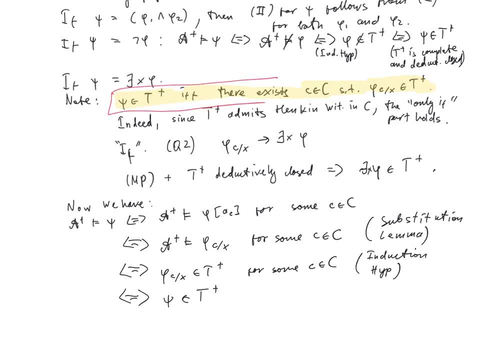 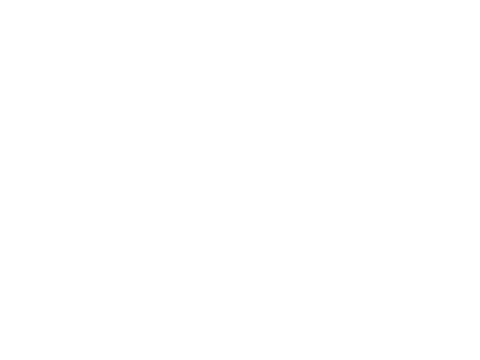 aforementioned observation. Now we are going to the proof of the completeness theorem. So next we have the following lemma: For any consistent L-theory, there exists a set of constant symbols. So this is the property of the constant symbols: c disjoint from the language L. 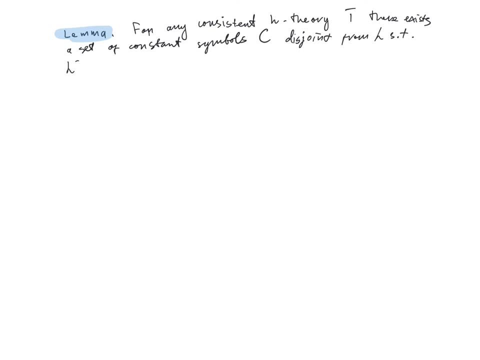 Such that if we take L plus to denote the language L union, c, Then there exists a complementary example: a constant symbol A plus is just like a constant symbol c. It's the corresponding complete L plus theory, T plus, which contains T, and so that T plus admits Henkin witnesses. 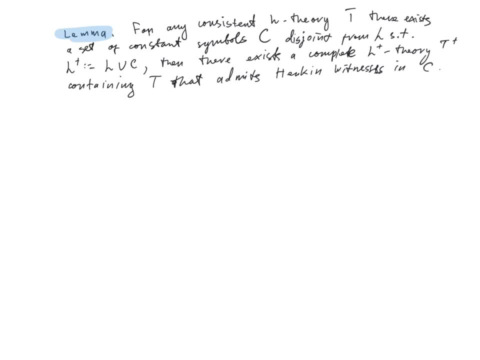 In C. So this lemma says that, starting with anial theory, which is consistent, we can find a set of constant symbols all disjoint from the language, and we can find an expansion T plus of our theory, T that now has Henkin witnesses in this new set of constant symbols C. 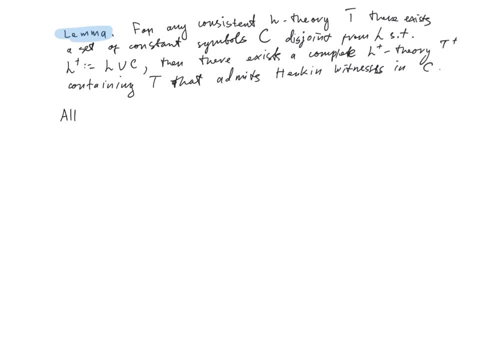 Before proving this lemma, let us observe that this lemma allows us to conclude the proof of the completeness theorem. Indeed, if A plus is a model of the L plus equal to L, union C theory: T plus with T plus containing T, then the reduct of the L plus structure A plus to the language L is, in particular, a model of T. 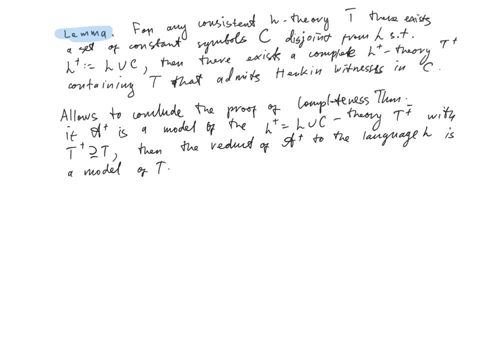 And so, assuming we're given some consistent L theory T, using this lemma we can extend it to a theory T plus in the language L plus, which admits Henkin witnesses in C and is complete. Hence we can apply proposition 1 to demonstrate that T plus admits a model. 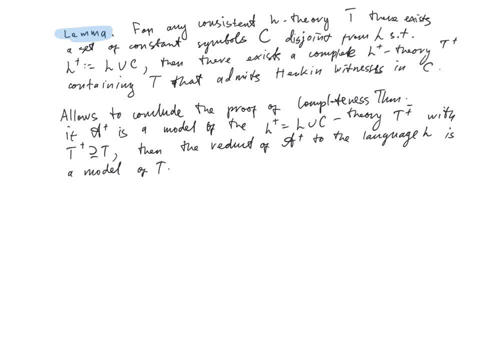 And by this remark, any model for T plus. once we consider it, we can apply proposition 1 to demonstrate that T plus admits a model If we consider that T plus is a subset of the previous proof, if we consider its reduct to the sub-language, L is a model of T because T is a subset of T plus.